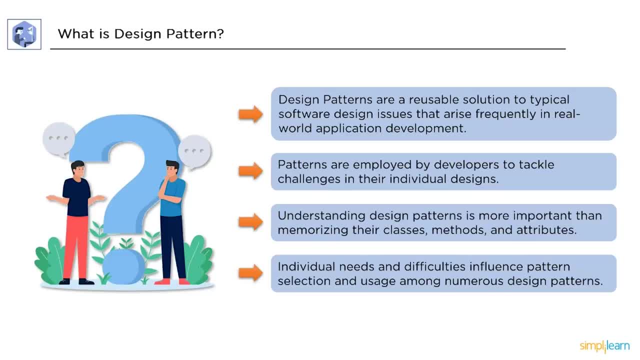 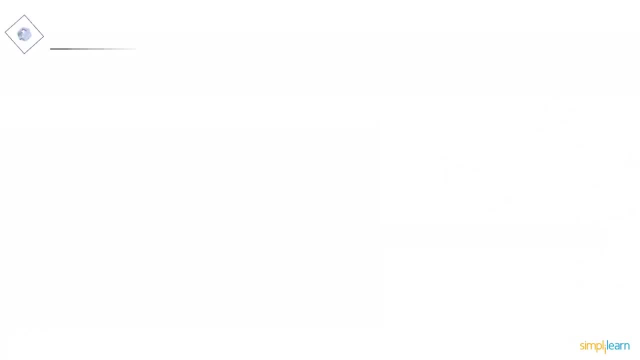 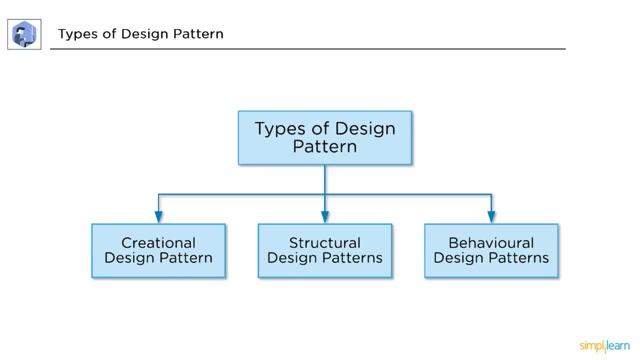 and usage among numerous design patterns. Now let's discuss types of design pattern. There are three types of design patterns available: Creational design pattern, structural design pattern and behavioral design pattern. Let's start with creational design pattern. The creational design patterns deal with object. 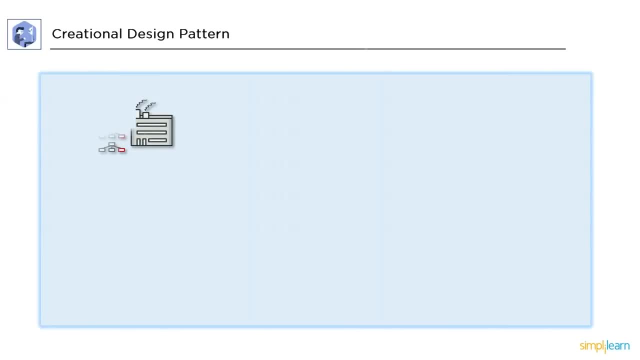 creation and initialization. A creational design pattern gives the�iss try with a с which designers will use this drums. We have 5 kinds of design patterns: Fabs, Tracks, Builders, Statuser. Let's discuss each of them in detail. 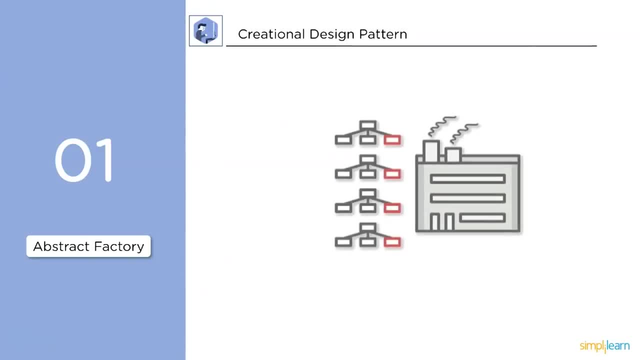 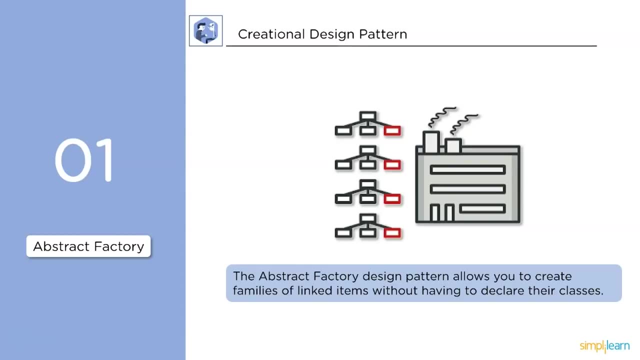 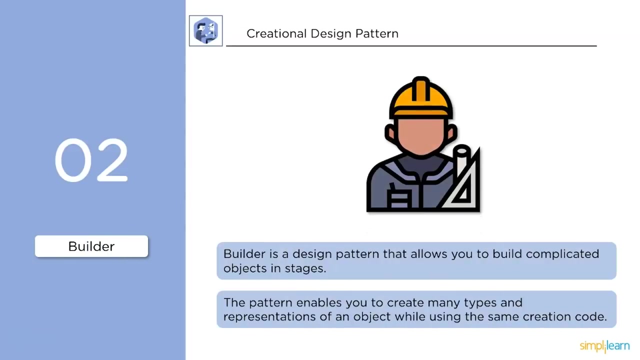 First up, Abstract Factory. The Abstract Factory design pattern allows you to create families of linked items without having to declare their classes. Next up, Builder Pattern. Builder is a design pattern that allows you to build complicated objects in stages. This pattern enables you to create many types of representations of an object while using the same creation code. 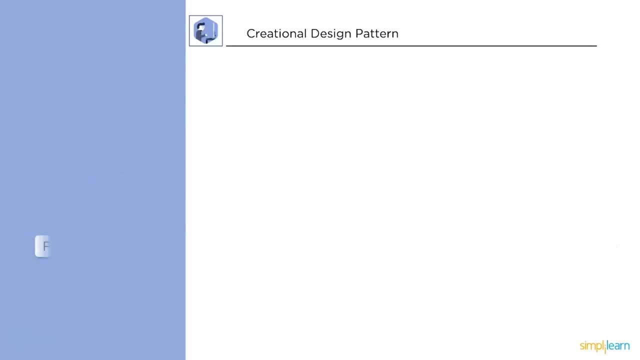 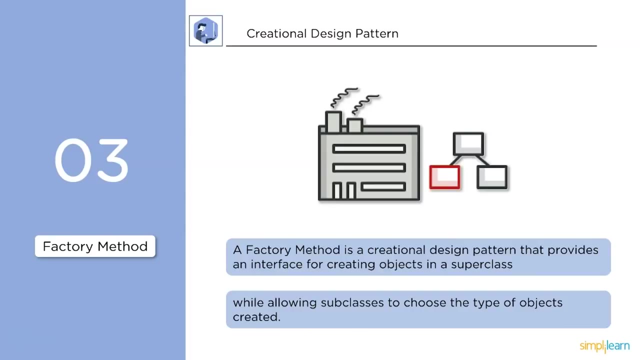 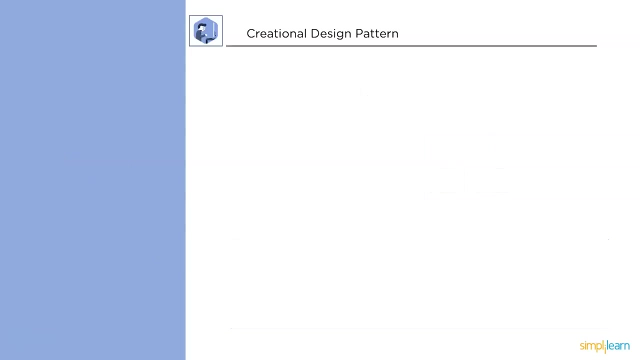 Next up: Factory Method. A Factory Method is a creational design pattern that provides an interface for creating objects in superglasses, while allowing subclasses to choose the type of object created. Next up: Prototype: Prototype pattern is a design pattern that allows you to create multiple types of objects. 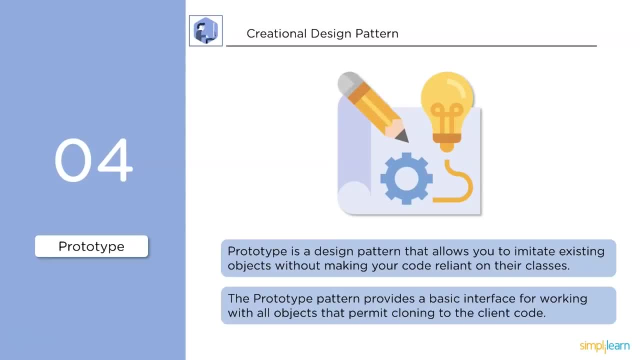 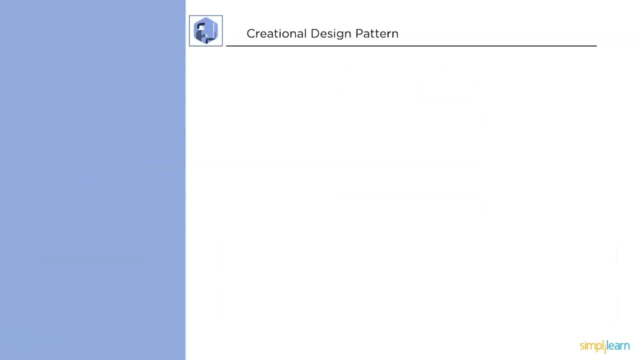 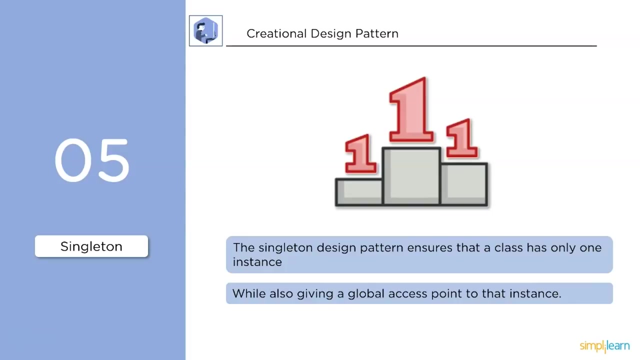 This is a design pattern that allows you to imitate existing objects without making your code land on their classes. The Prototype pattern provides a basic interface for working with all objects that permits cloning to the client code At last. Singleton: The Singleton pattern ensures that a class has only one instance while also giving a global access point to that instance. 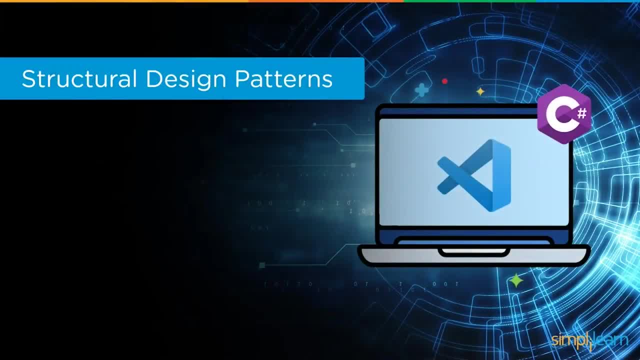 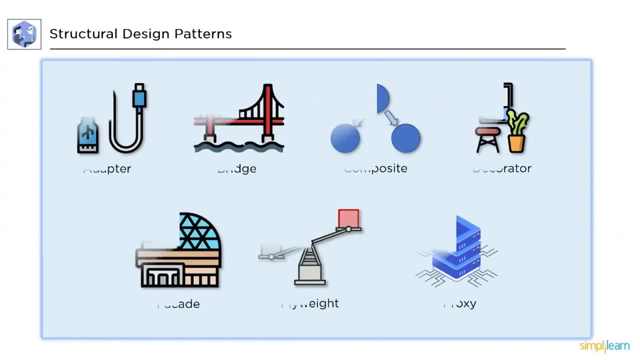 Next up, Let's discuss the Structural Design Pattern. The Structural Design Pattern is basically used to manage the structure of classes and interfaces, as well as manage the relationship between the classes. We have seven types of design patterns in this: Adapter, Bridge, Composite Pattern, Decorator Pattern, Facade Pattern, Flyweight Pattern and Proxy Pattern. 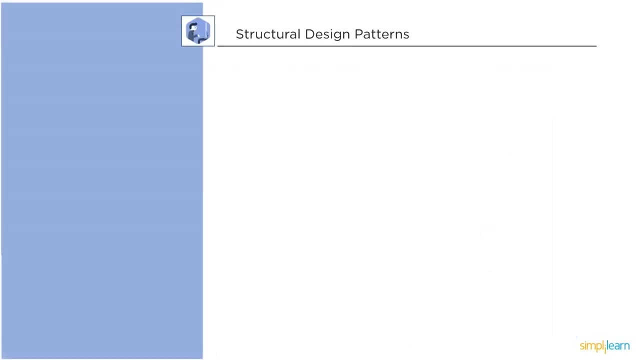 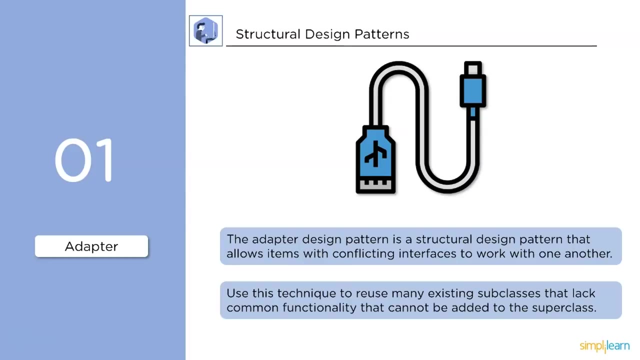 Let's discuss each of them in detail. First up, Adapter. The Adapter design pattern is a structural design pattern that allows items with conflicting interfaces to work with one another. We use this pattern to reuse many existing subclasses that lacks common functionality that cannot be added to the superclass. 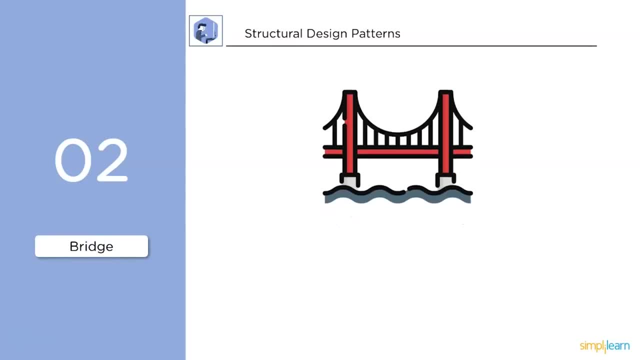 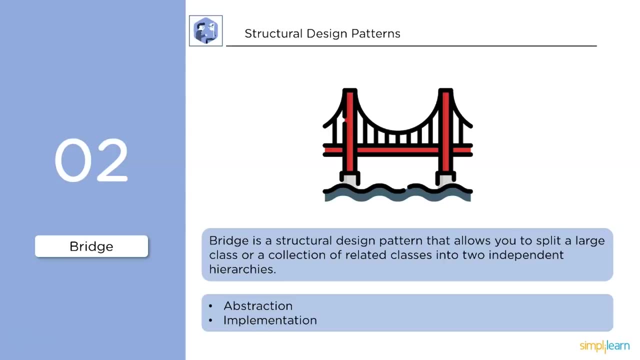 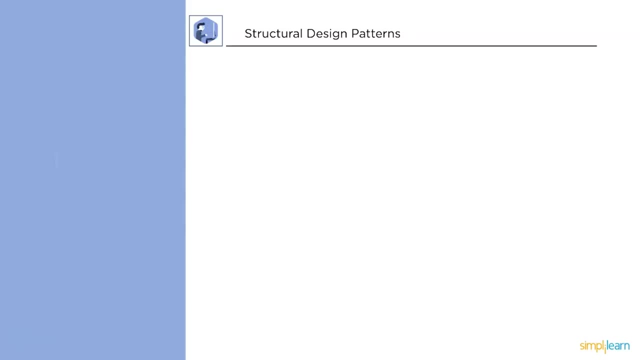 Next up, Bridge. Bridge pattern is a structural design pattern that allows you to split a large class or a collection of related classes into two independent hierarchies: abstraction and implementation. Next, Composite Pattern. Composite is a structural design pattern that enables you to organize parts into three structures. 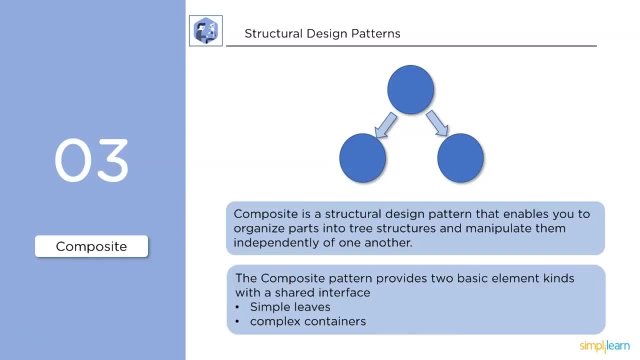 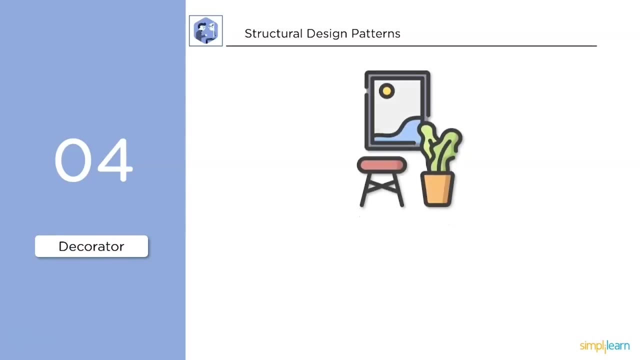 and manipulate them independently of one another. The Composite pattern provides two basic element kinds with a shared interface: simple leaves and complex containers. After that, Decorator: Decorator is a structural design pattern that allows objects by wrapping them in a special wrapper. object: 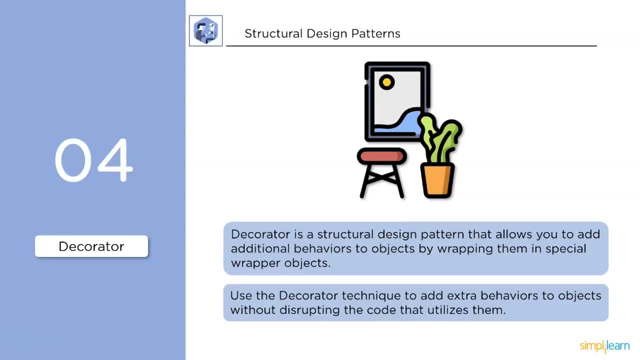 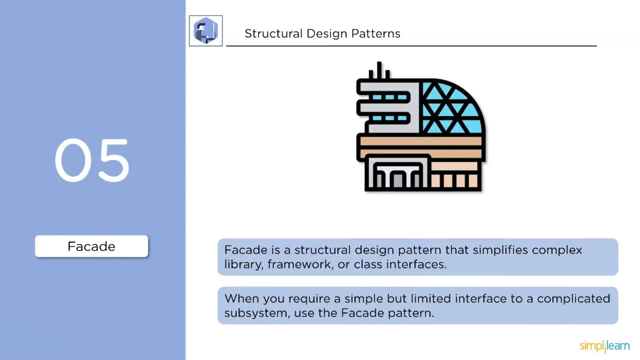 This pattern uses the decorator technique to add extra behaviors to objects without disrupting the code that utilizes them. Next up, Facade. Facade is a structural design pattern that simplifies complex libraries, frameworks and class interfaces When you require a simple but limited interface to a complicated subsystem. 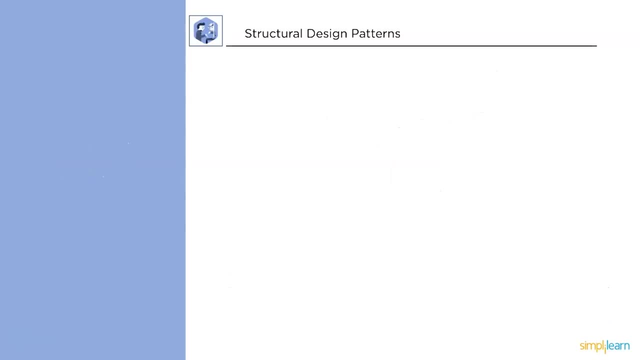 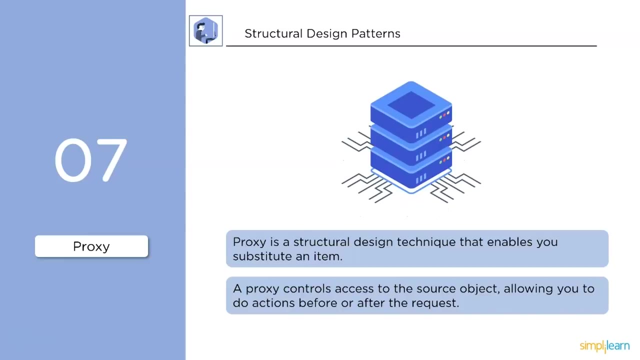 we use the Facade pattern At last. Proxy Pattern. Proxy is a structural design pattern that enables you to substitute an item. A proxy controls access to a source object, allowing you to do actions before or after the request. Next up is a behavioral design pattern. 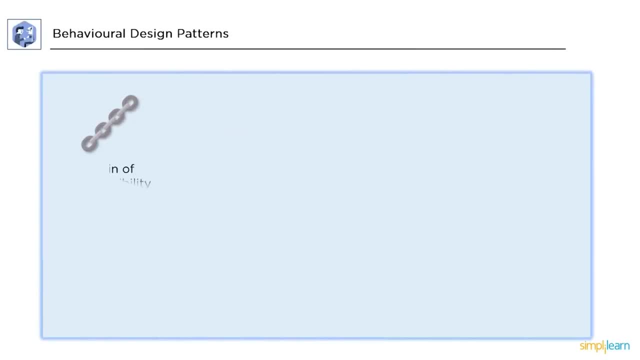 The behavioral design pattern deals with communication between classes and objects. That means if you want to change the behavior of a class and again you want it to affect other classes of the project as well. We have 10 types of design patterns available in this. 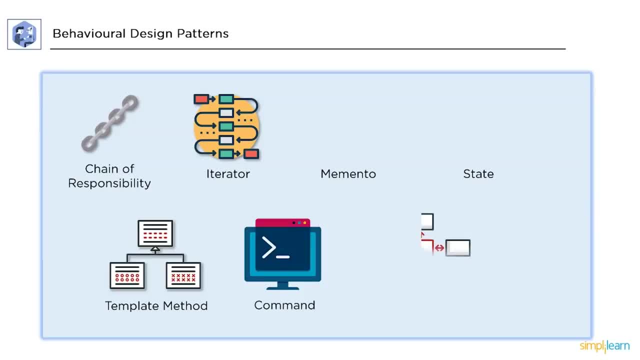 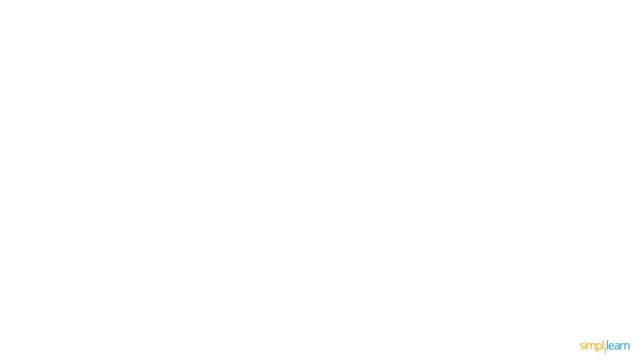 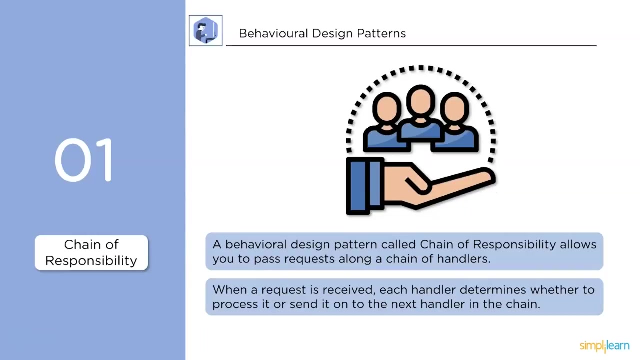 Chain of Responsibility, Iterator, Memento, State, Template, Method, Command, Mediator, Observer, Strategy and Visitor. Let's discuss them in detail. First up the Chain of Responsibility, A behavioral design pattern called the Chain of Responsibility allows you to pass requests along the chain of handlers. 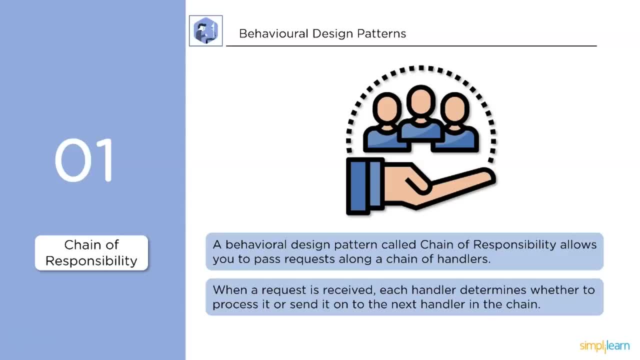 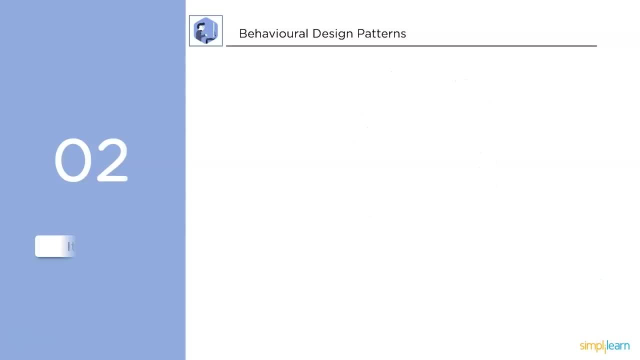 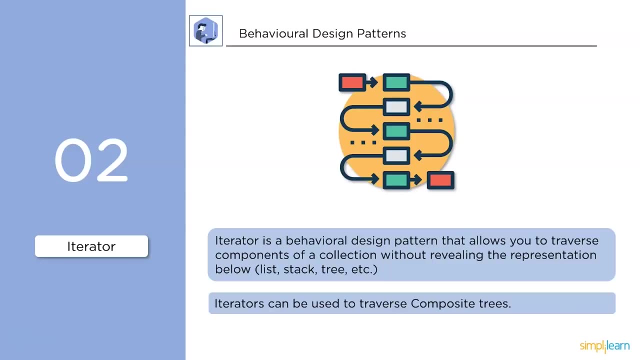 When a request is received, each handler determines whether to process it or send it to the next handler in the chain, Next up Iterator. Iterator is a behavioral design pattern that allows you to pass requests along the chain of handlers. It allows you to traverse components of a collection without revealing the representation below. 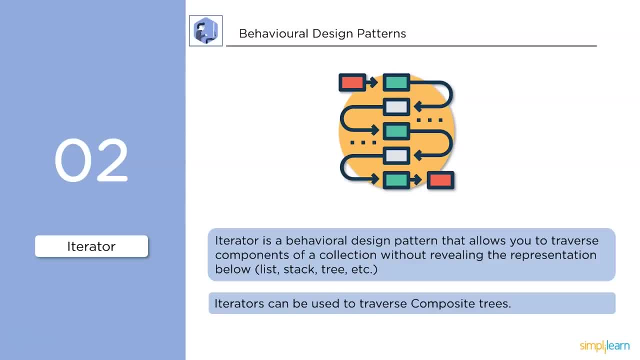 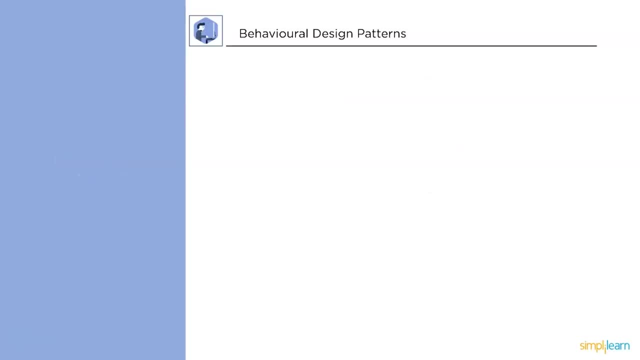 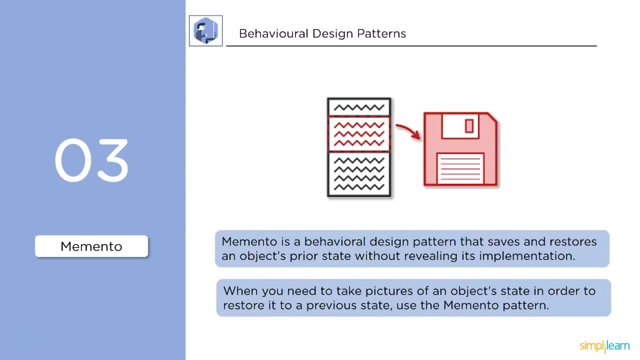 That is, list, stack, tree, etc. Iterators can be used to traverse composite trees. Next up is Memento. Memento is a behavioral design pattern that saves and restores an object prior state without revealing its implementation. When you need to take pictures of an object's state in a project, you can use the Memento. 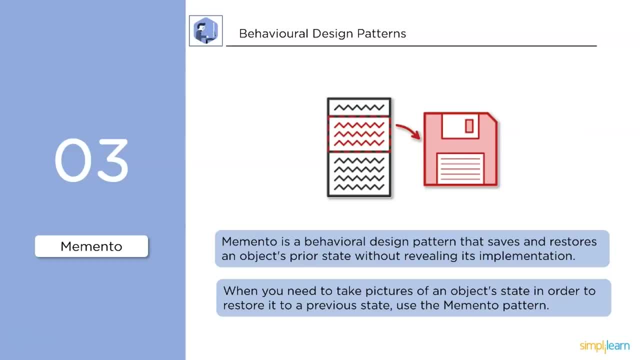 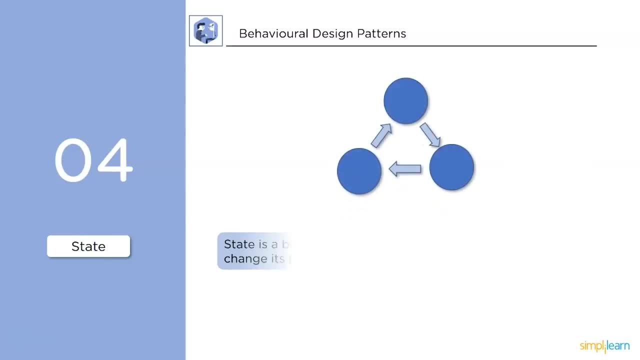 To restore an object's state. in order to restore it to a previous state, we use Memento pattern, Next up State Pattern. State is a behavioral design pattern that allows an entity to change its behavior in response to the changes in its internal state. 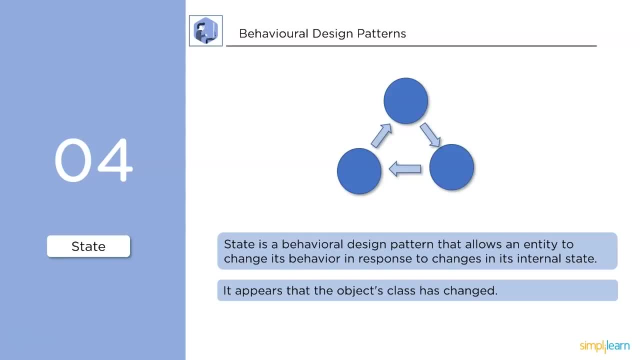 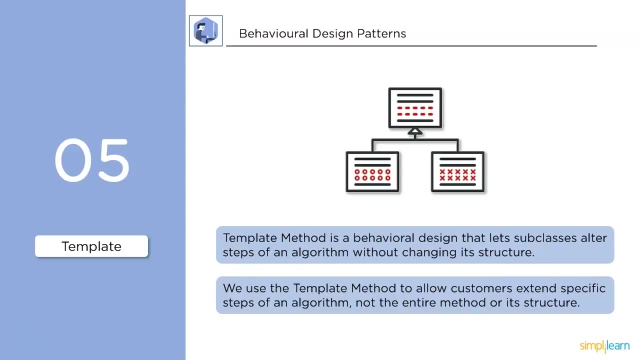 It appears that the object's class has changed, Then the Template Pattern. Template Method is a behavioral design that lets subclasses alter steps of an algorithm. We use the template method to allow customers to extend specific types of an algorithm, not the entire method or its structure. 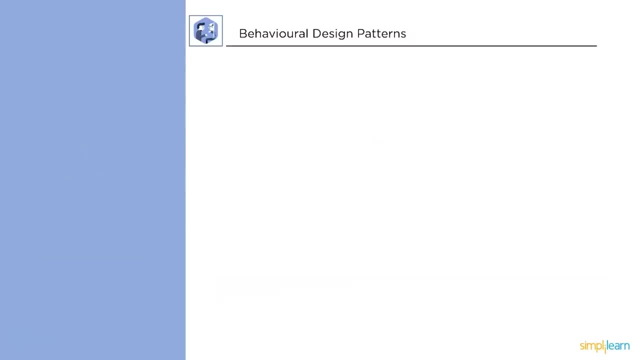 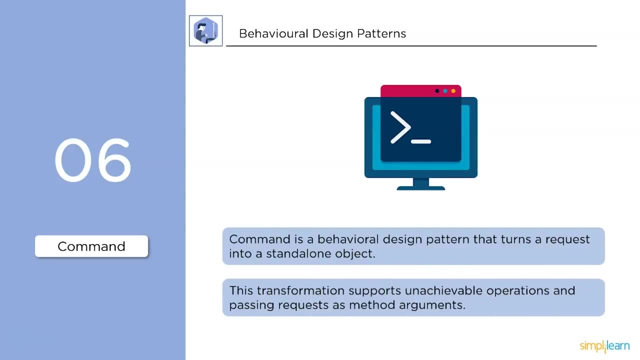 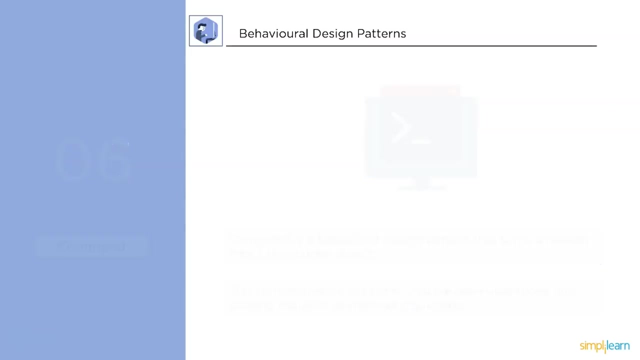 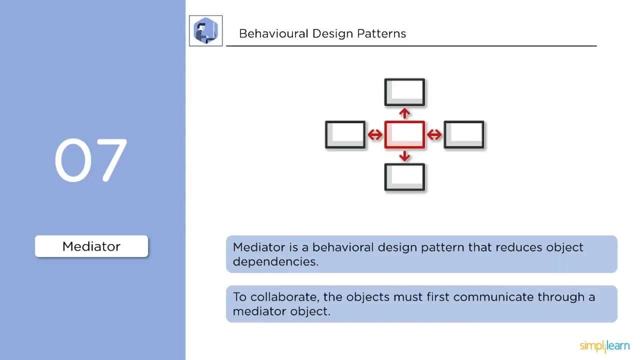 Then we have Command Pattern. Command is a behavioral design pattern that turns a request into a stand-alone object. This transformation supports unachievable operations and passing requests as method arguments After that Mediator. Mediator is a behavioral design pattern that reduces object dependency. to collaborate, the objects must first communicate to a mediator. object: 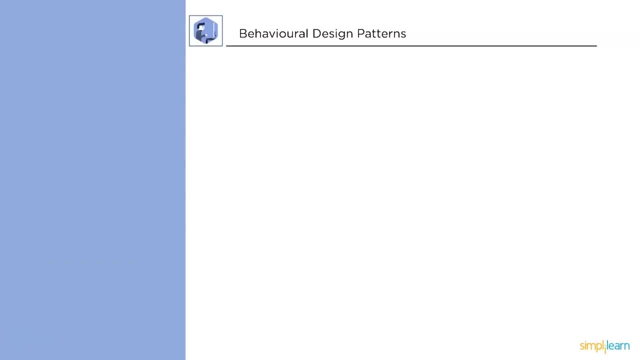 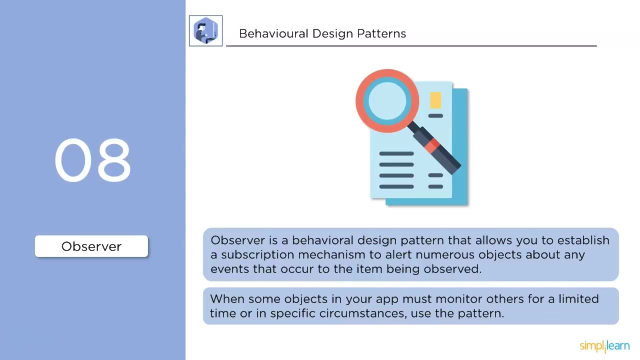 Next up is Observer Pattern. Observer is a behavioral design pattern that allows you to establish a subscription mechanism to alert numerous objects about an event that occurred to the item being observed. When some objects in your app must monitor others for a limited time or in specific circumstances, we use this pattern. 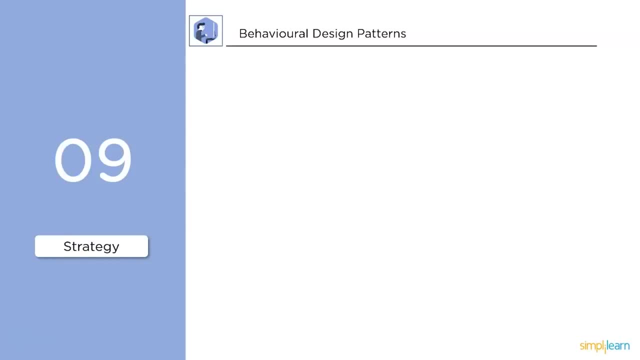 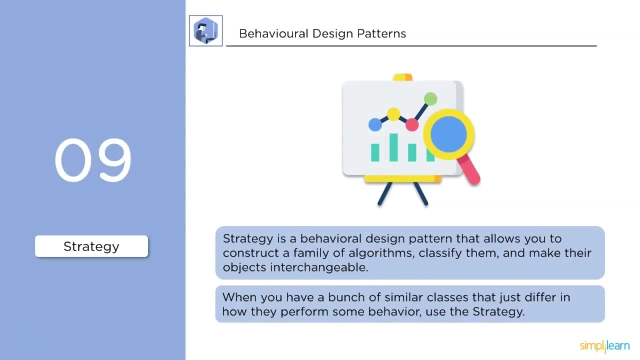 Next up, Strategy Pattern. Strategy is a behavioral design pattern that allows you to construct a family of algorithms, classify them and make the object interchangeable. When you have a bunch of similar classes that just differ in how they perform some behavior, then we use the Strategy Pattern. 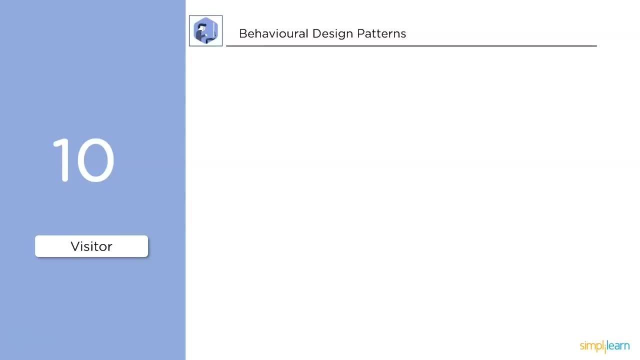 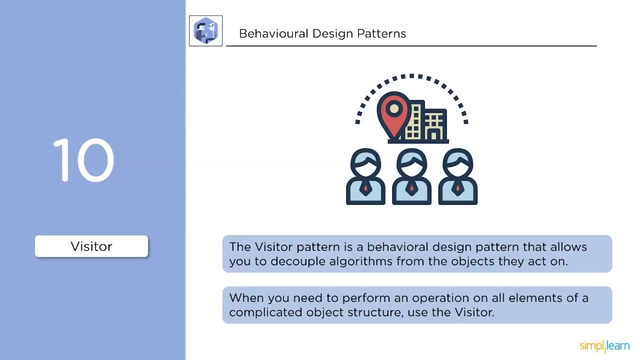 At last, Visitor. The Visitor Pattern is a behavioral design pattern that allows you to decouple algorithms from the objects they act on. When you need to perform an operation on all elements of a complicated object structure, we use the Visitor. Finally, let's conclude this tutorial with some advantages of design patterns. 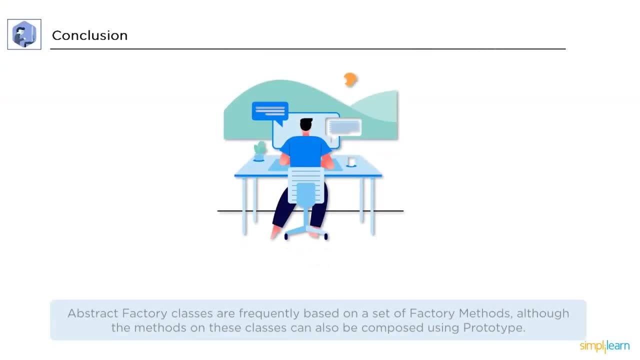 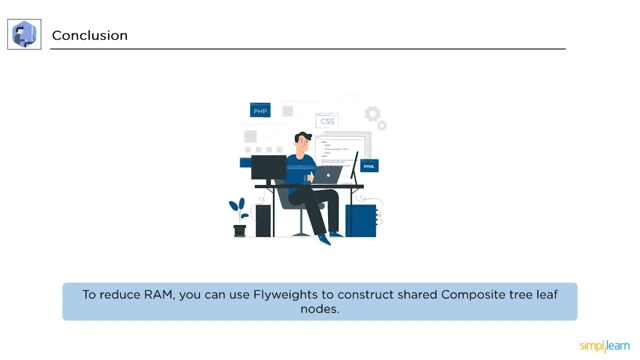 First up, Abstract Factory Classes. Abstract Factory Classes are frequently based on a set of factory methods, although the method on these classes can also be composed using a prototype. Next up, to reduce RAM, we can use fly weights to construct shared composite tree leaf nodes. 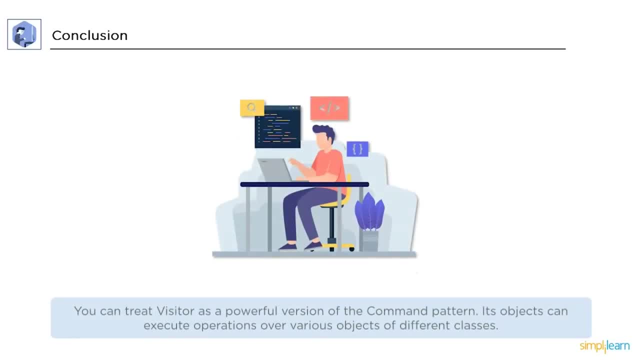 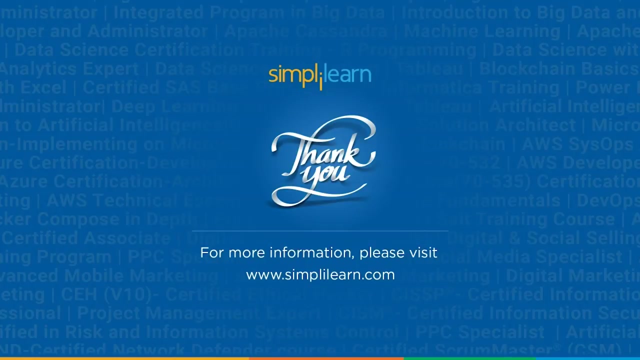 Finally, you can treat a visitor as a powerful version of the Command Pattern. Its objects can execute operations over various objects of different classes. And this was all for today's session. Hope you guys found it informative and helpful. If you liked this session, then like, share and subscribe. 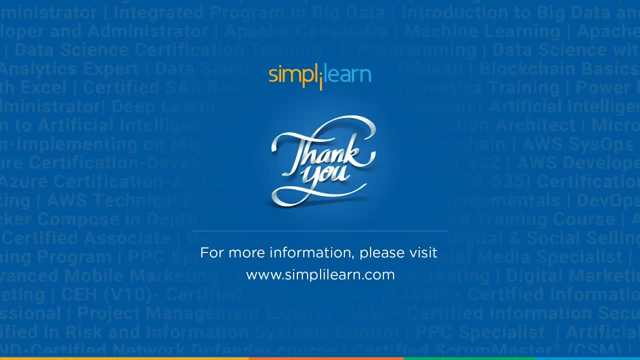 If you have any questions, then you can drop them in the comment section below. Thanks for watching and stay tuned for more from Simply Learn.